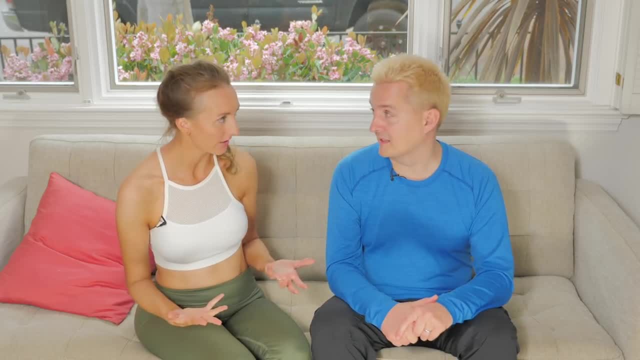 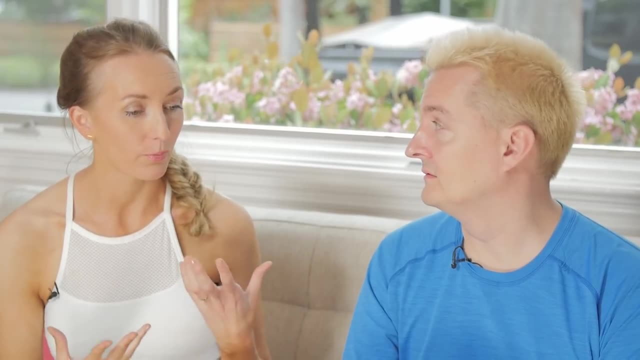 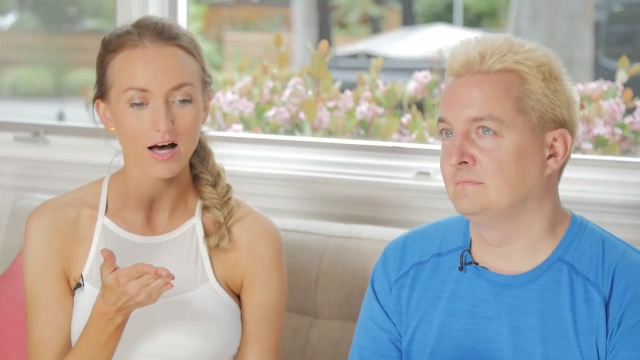 and then in for five and out for five. But it's great to start even just with one, two, three. one, two, three. Then you can work to add what's called a gentle breath retention or a pause at the top. So inhale for one, two, three through the nose, pause. 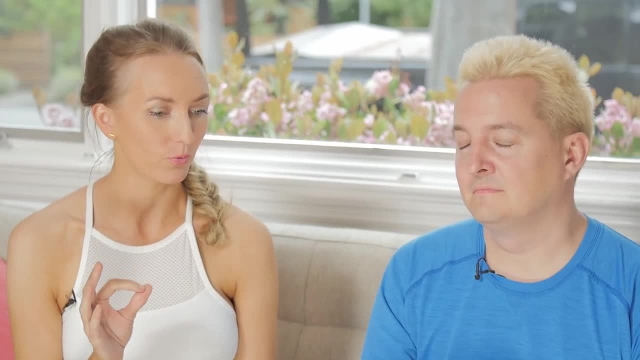 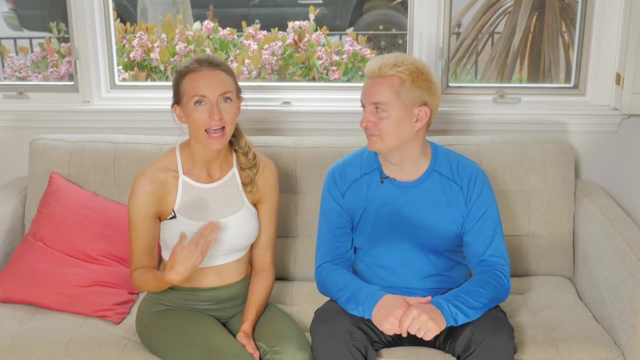 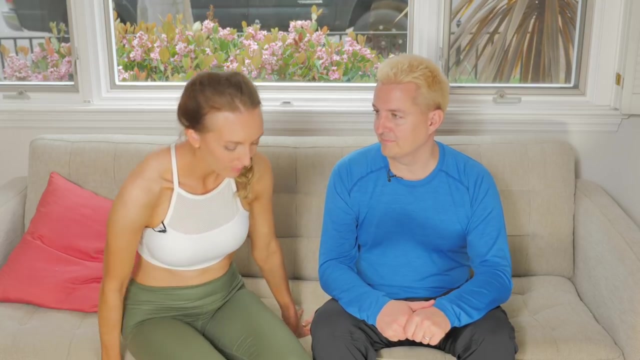 exhale three, two, one through the nose. pause. Do you already feel calmer? Yes, It just slows you down. Slows you down So you can start to add that pause. The other thing I talked about here was the idea of a full, complete breath. So in order to help Murray really find that, 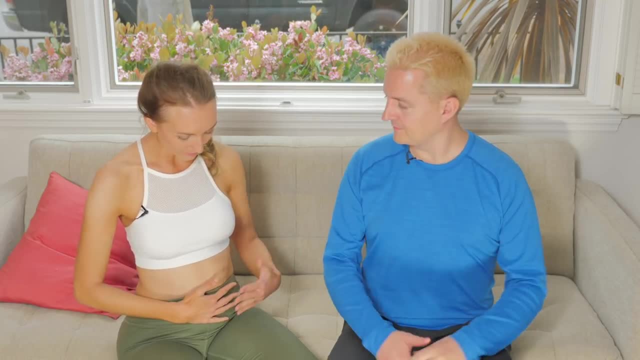 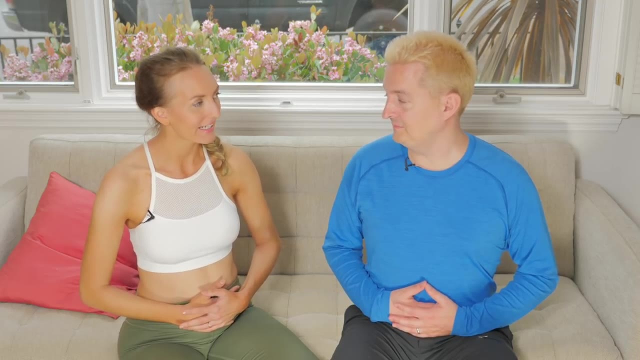 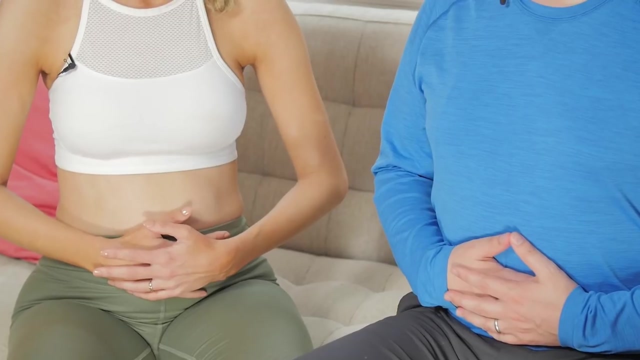 I'm going to have him come to the edge of his seat- So he's sitting nice and upright- and just take both hands to his navel. And this is a fun game. Basically, we're going to inhale and we're going to see if your navel moves or not. So inhale and exhale. 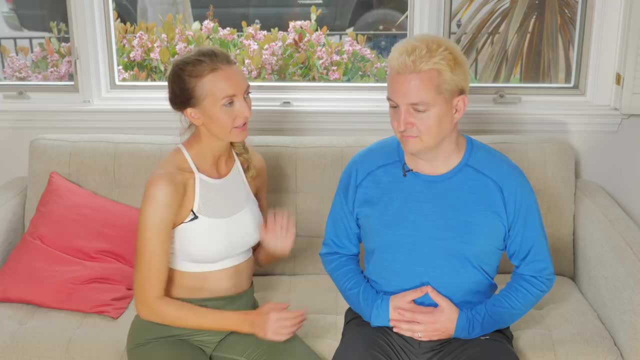 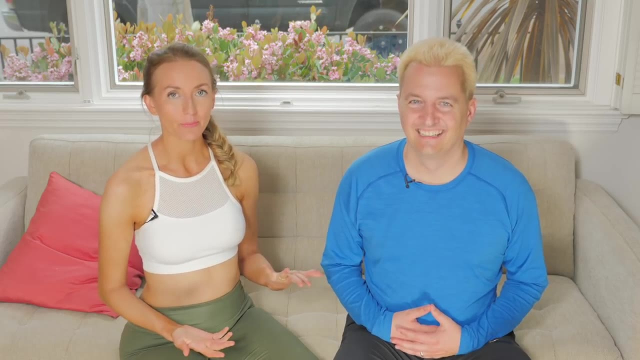 So all of his breath that you guys see was in his chest. Do it again, Murray, Breathe in. Okay, You fixed it that time. He fixed it, He knew. So the first time he took a breath, I saw because I was looking at his navel underneath his hands and his navel didn't move. 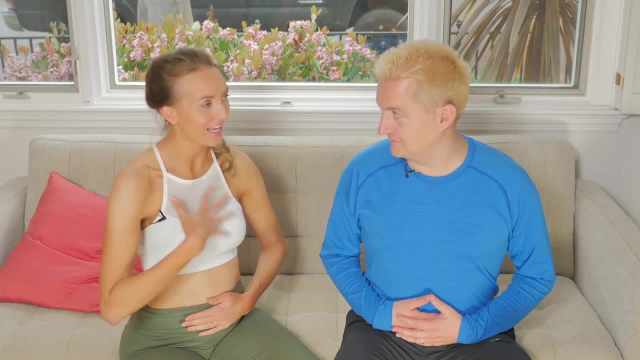 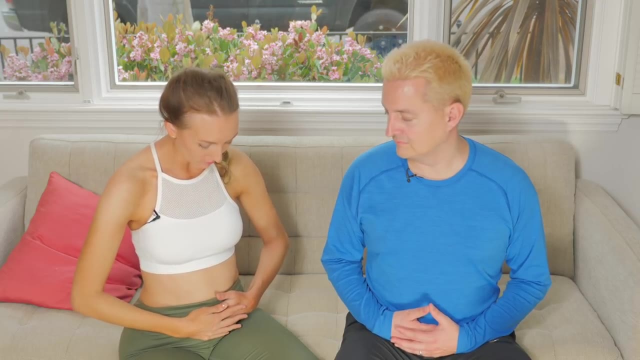 He breathed like this: It was just up in the upper body. Yeah, What we want to do when we breathe in yoga is send the breath all the way down so that your navel actually moves out, And then, when you exhale, the navel moves in. 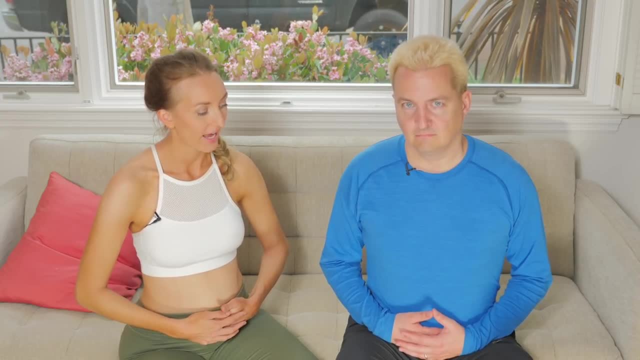 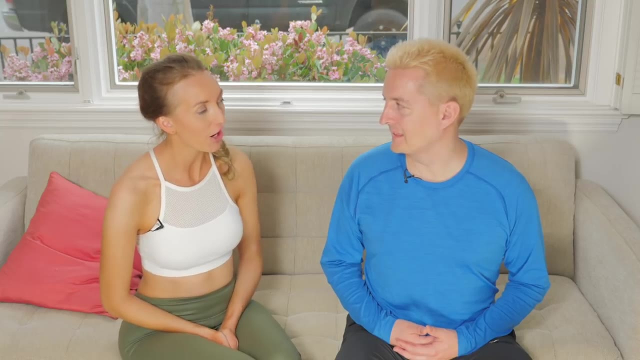 Try that one more time: Inhale, exhale, So you have a deep belly breath, a full, complete breath. And this is really hard because so many of us are used to our whole life just breathing up here in our chest. Yeah, 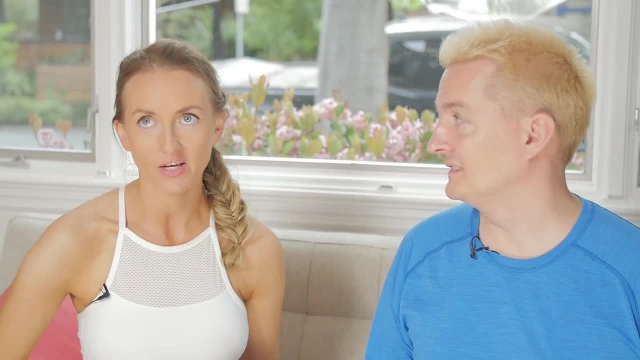 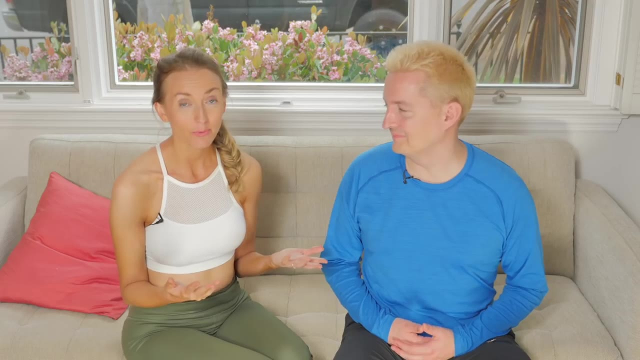 And a lot of us also are self-conscious about this area of the body We're constantly sucking our belly in, And a fun anecdote I like to share is that if you've ever seen statues of Buddha, Buddha is big, Has a big belly- 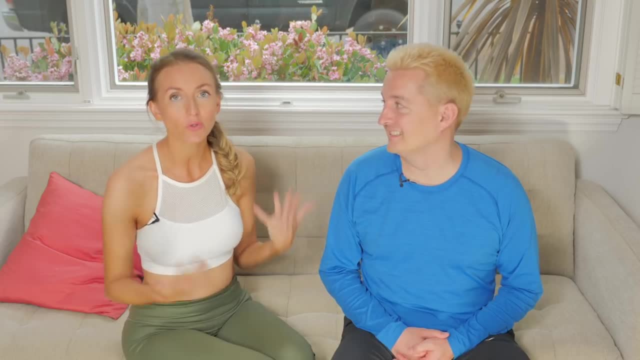 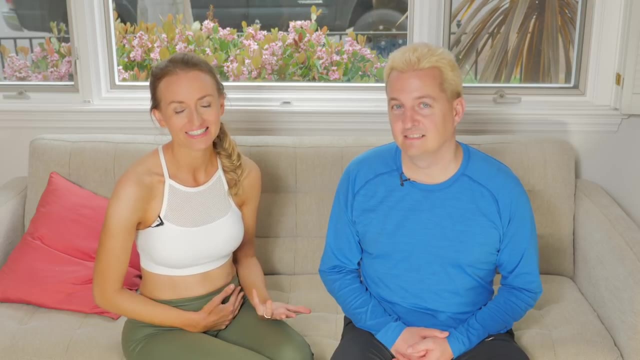 He's got a big belly And the reason is because he was a master meditator and he knew how to send his breath down into his body. Interesting, Yeah. So we need to reclaim awareness of this area, of the solar plexus area. And as you breathe, 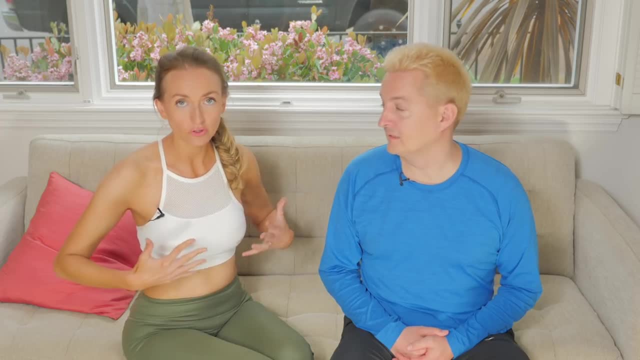 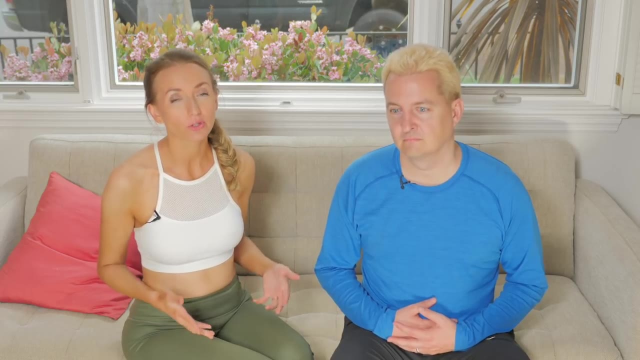 you want to think of what's going on in your body. You want to think of what's going on in your body, So you need to be aware of really sending the breath into the whole ribcage. So that means that your diaphragm is going to really contract and then release with each breath, And that is going. 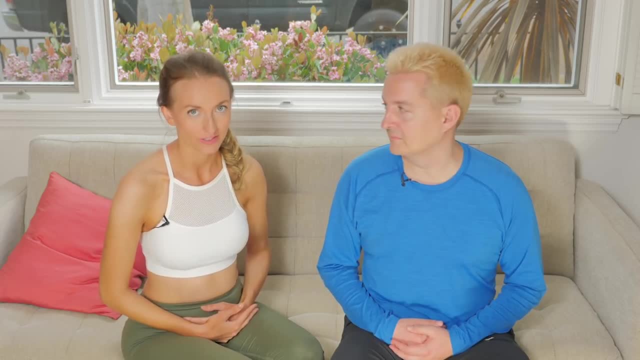 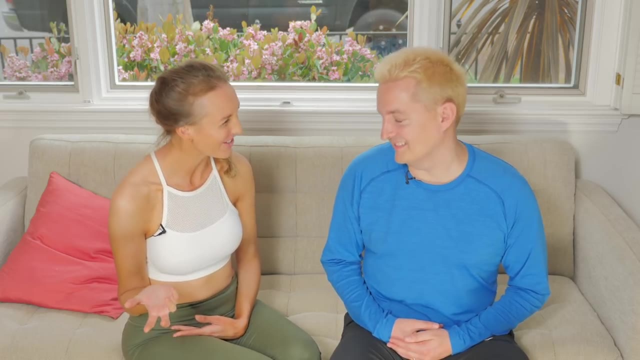 to push the navel out, And that's okay. That's okay. We want those full, deep, complete breaths, especially as a beginner, because even if you're not doing some of the postures, quite right because you're new to yoga- if you can do the breathing right, you're going to get. 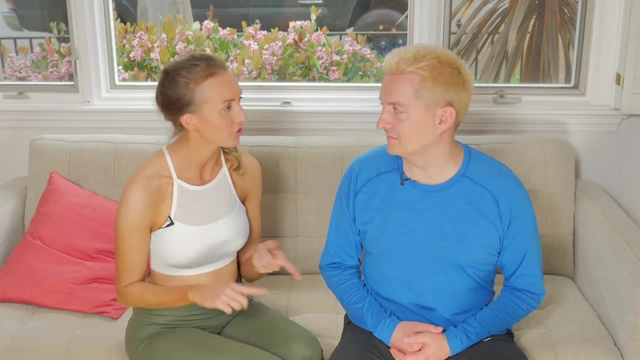 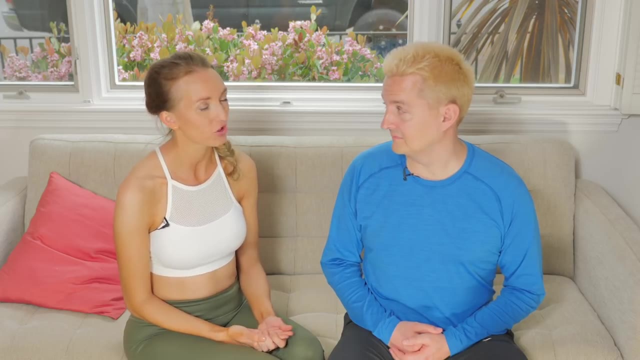 so many of the benefits of this practice: the stress reduction and everything, everything that comes with it. Now, once you're comfortable with this, there's something called Ujjayi Pranayama, which I have a different video on. 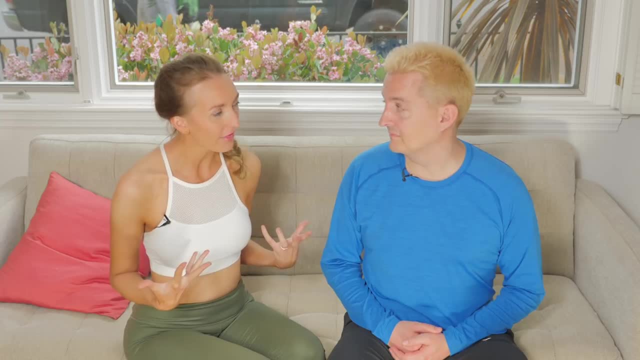 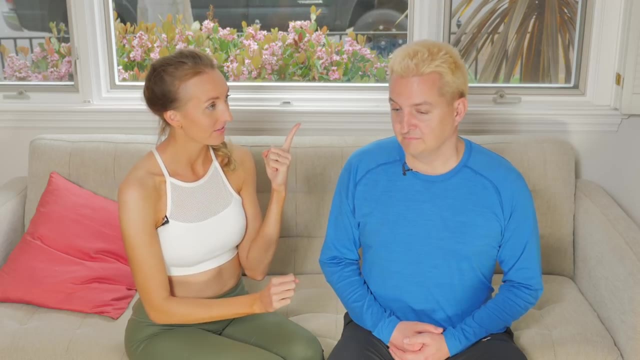 which is sort of the traditional, more heating, yogic breath. But if you are just starting out, this is the way to go. Just focus on- let's recap- Inhales from where Murray? From the mouth, from the nose, from the nose. 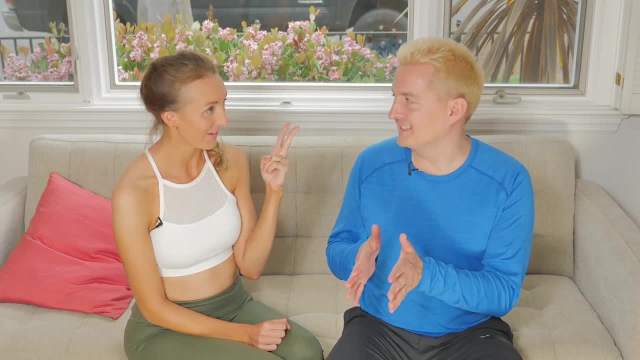 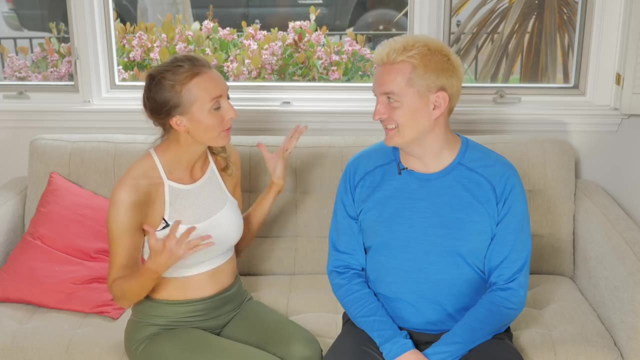 In and out through the nose For the same length of time. in and out, Perfect. and the third thing: Counting to three in, counting to three out, Counting to three in and out, and yeah, and just trying to keep that full, complete breath. 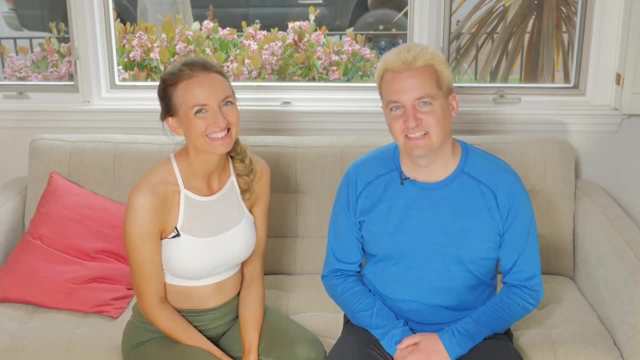 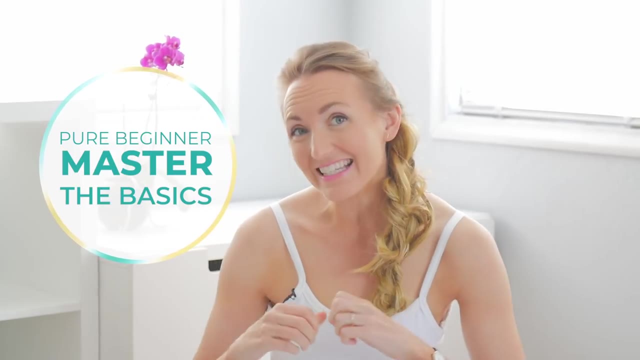 Yeah, in and out You got it. We'll see you guys in the next video. See you next time. Hey, if you liked this video, you are going to love my free, pure beginner master the basics yoga class. Not only do I cover the top 10 yoga poses, 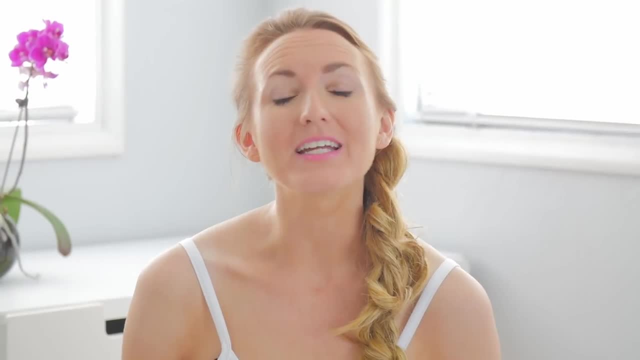 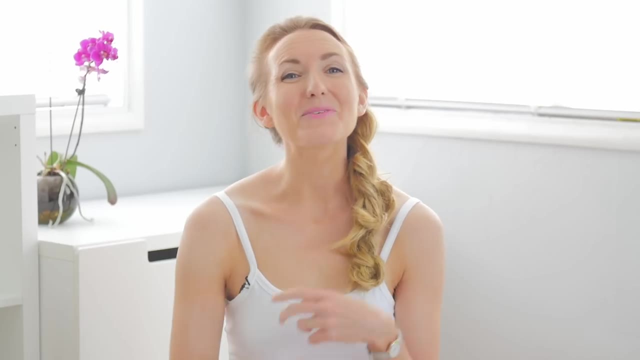 you're most likely to encounter as a beginner, but I give you a downloadable cheat sheet showing you exactly how to do each of these moves, so you know you're doing them correctly. Let's banish the fear and confusion of doing it wrong. Let's master the basics together. 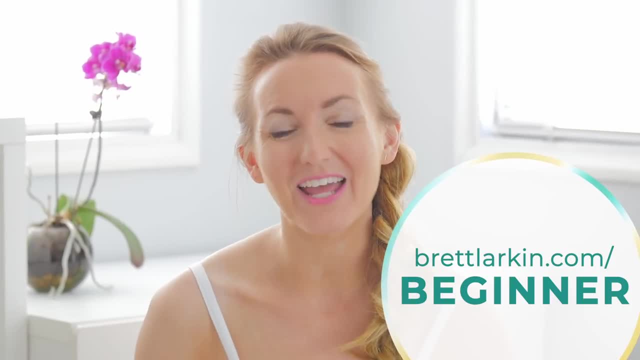 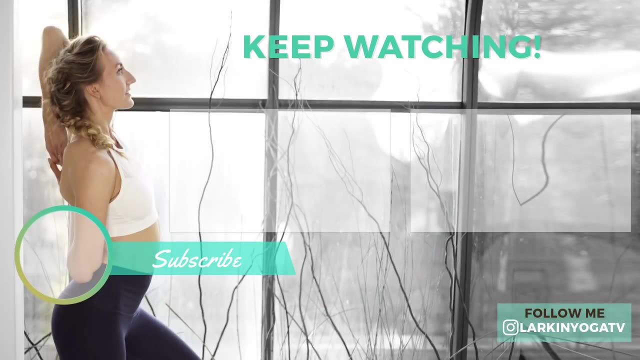 Go to brettlarkincom, forward, slash beginner for your free download and I'll see you on the mat. Namaste, Namaste.